got to take antibiotics for tuberculosis for 6 to 12 months because it's such a slow organism. well, these organisms kind of turn down their metabolism when they're hiding in a biofilm. so number one: they're just much harder to kill with antibiotics or anything else. number 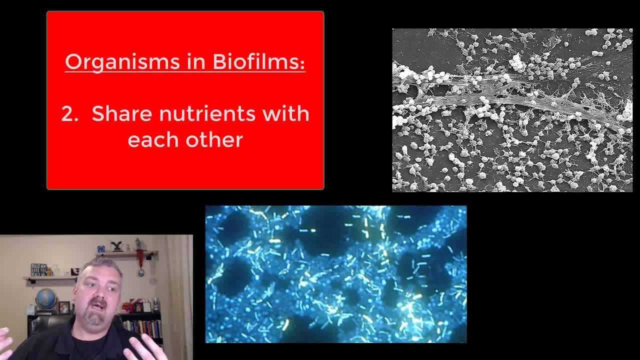 two, while they're in there, they're sharing nutrients. think about like: so basically, the organisms that use oxygen are creating an anaerobic environment for the ones that don't want oxygen, or the ones that the ones that produce methane gas are feeding the ones that like methane gas and all these kinds of things. so basically, the waste products or byproducts. 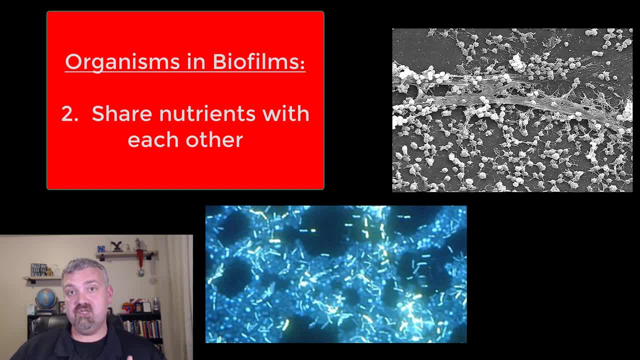 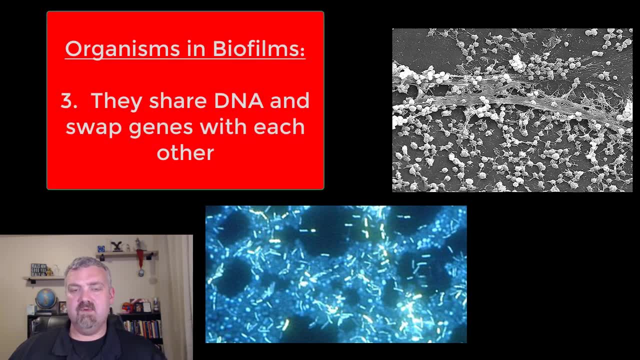 of one organism become the food of another. so they're sharing nutrition and food, making them healthier. They're also they're hiding. they're sharing food, But they're also sharing DNA. So imagine the amount of horizontal gene transfer, or genetic swapping, that occurs inside a biofilm. 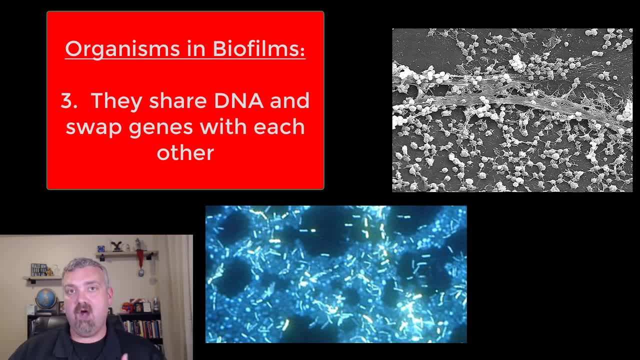 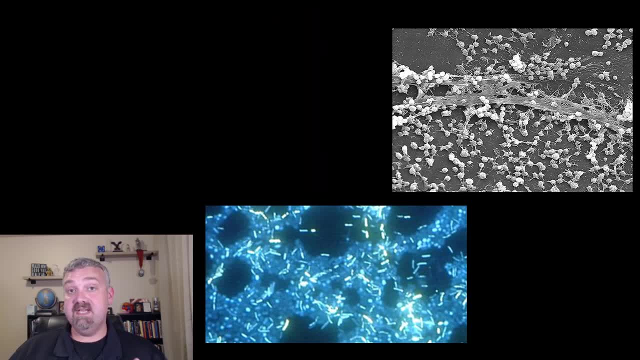 So when organisms come out of a biofilm, they are generally heartier and more dangerous than when they went in, So that's why they're so significant. The other reason I'd say they're very, very significant is if you're dealing with a biofilm. 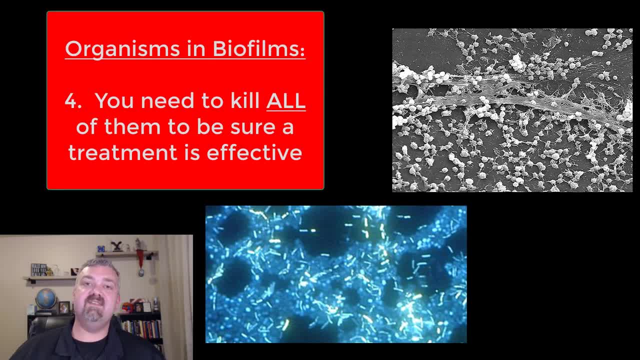 infection if you don't kill all of them. killing ninety nine percent of the organisms hiding in a biofilm is not enough, because they will just quickly come back. The best two examples I can give you would be, You know, persistent chronic urinary tract infection. 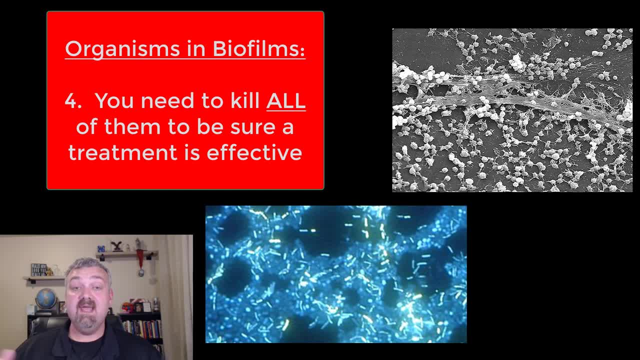 So if you ever had a patient that has a UTI every four weeks, every six weeks, whatever, they have one, right, They have one UTI you treat with antibiotics. It kills as many of the cells as it can to to control the symptoms. But since you can't, didn't eradicate the biofilm, didn't eradicate all the organisms living. 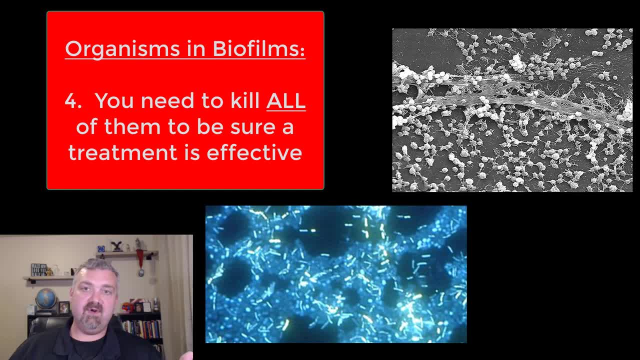 in it. they just pop back up. So four weeks later it's the same urinary tract infection. It's just you're. you're hammering it down, It pops back up. Another example would be strep throat. Like people that have strep, 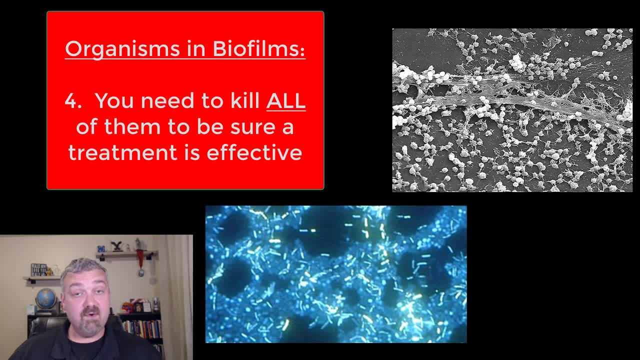 Once or twice every year until they get their tonsils removed, and then all of a sudden, they don't have strep very often, or maybe not at all. Well, you can make a very strong argument that there's a biofilm on the tonsils. that is that. 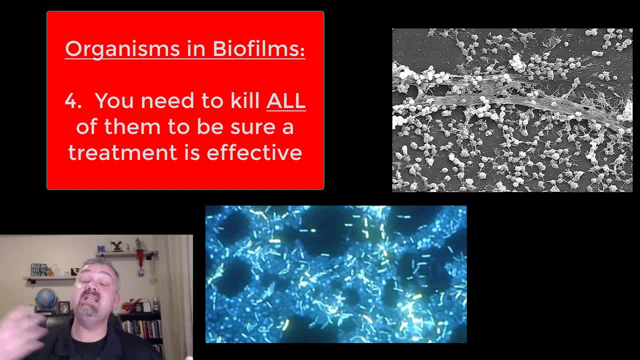 is a breeding ground for the strep infection. So you're actually physically removing the biofilm when you take somebody's tonsils out. Another example would be SIBO- small intestinal bacterial overgrowth. Studies have shown that you can put someone in antibiotics for like eight months and you